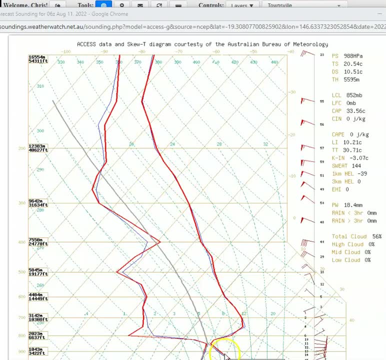 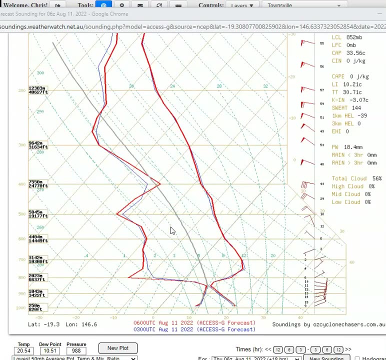 or a cross-section of what the atmosphere looks like from top to bottom over that location at that time of the day, And I'm not going to go into what soundings are. I have given you a link, or links down below, of tutorial series on how to read soundings, So if you're interested in becoming 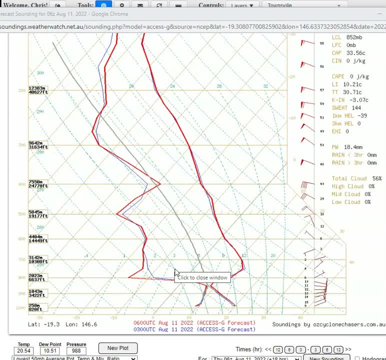 a bit more advanced in your weather, knowledge about soundings. please check out those links and work through those examples by having a real life one in front of you. The tutorial series will talk about what all these little letters and numbers are over here. Talk about what all these. 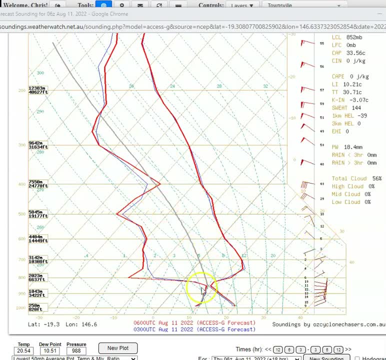 lines do and talk about what this represents, what this represents, what these lines represent. So all of that is done in the tutorial. No time to do that here? All right. so what we want to do, though, is we also want to understand that. you know, if we, if we look at a cross-section of the 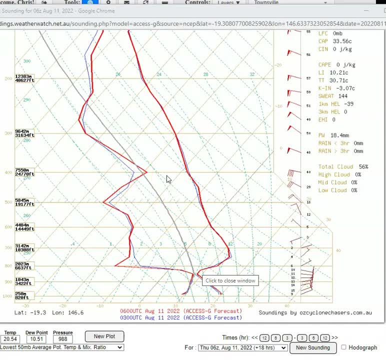 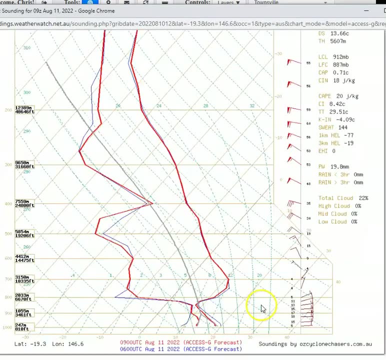 atmosphere at one point in time. it gives us an idea of what the atmosphere is looking like at that time. However, what we can do, then, is we can increase that by three hours. So, rather than looking at 4 pm, I want to look at 7 pm and see how the atmosphere is looking like at that time. 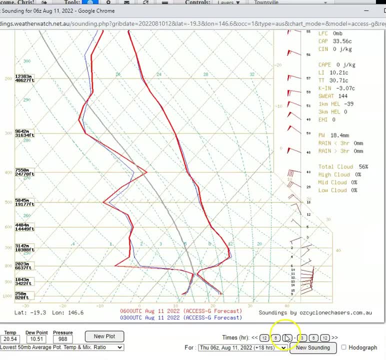 The atmosphere changes. or rather than looking at 4 pm, which is where we started, I want to look at 1 pm, So I can change the time frame that I'm looking at down here. So, rather than going back to the map and having to having to, you know, move that that model slider, we can do that here and we 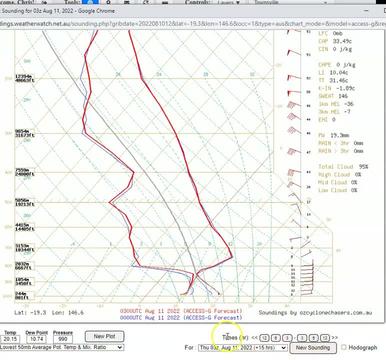 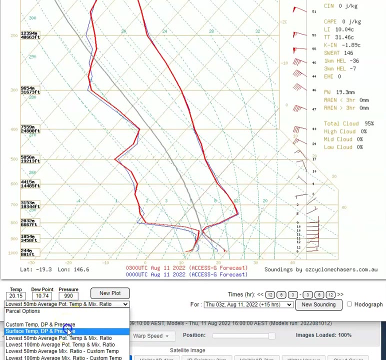 can go up in three hour, six hour or 12 hour increments. Now what also is interesting here is sometimes the computer models might get the surface temperature wrong. So let's say I can take two temperatures for the same temperature, the temperature for the two other temperatures. 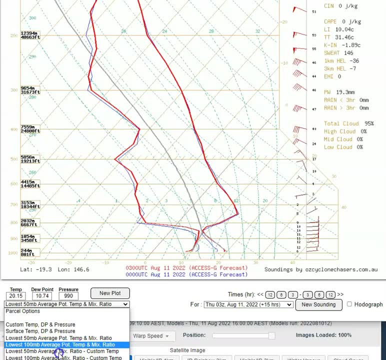 particularly the surface temperature is what I'd be interested in, because that's the one I know that can be, that can be wrong, Whereas the others, I'm sort of guessing these are a mixed temperature value and so these mixed temperature values they're pretty difficult to change without real 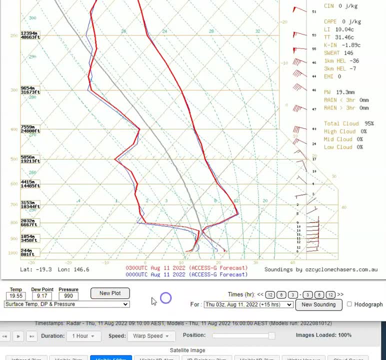 hard data. But if I say, let's say the, the model is saying that the temperature should be at at 1 pm today. it should be about 20 degrees where I'm am, But I've actually I've actually measured the temperature in my own weather station and it's about 6 degrees Fahrenheit and I've actually done a. 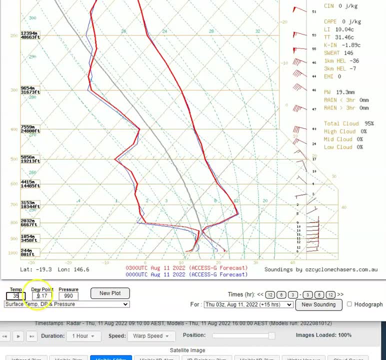 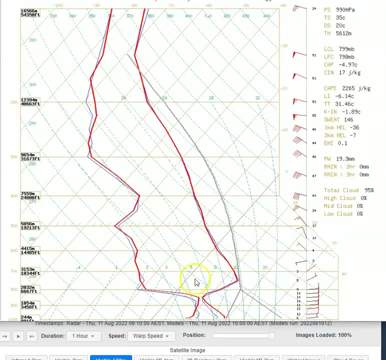 it's 35 degrees. So let's say it's 35 degrees and I've measured the dew point, and let's say it's 20 degrees. Now I can change those values and put in a new plot, and what that might do is it might. 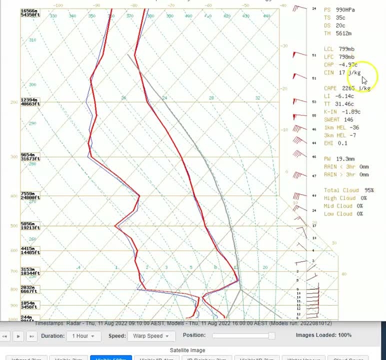 change a lot of these values. So see how these values have changed. Now. obviously in the real world you're probably not going to get that big a difference right between the actual temperature and the temperature that the model does. But sometimes those extra couple of degrees that 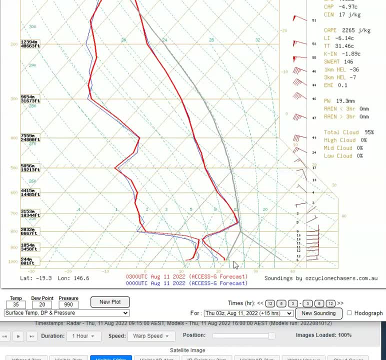 might heat up, and what we do know from our computer model data is that computer models do tend to under represent maximum temperatures, And so what we can do, then, is we can replot the same scenario in the in the rest of the atmosphere, but just changing the surface parameters can change. 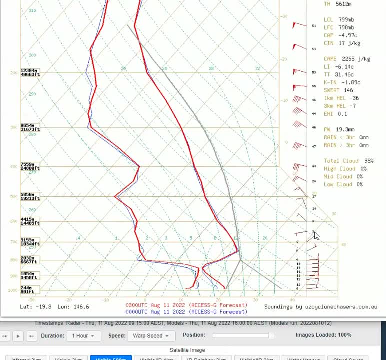 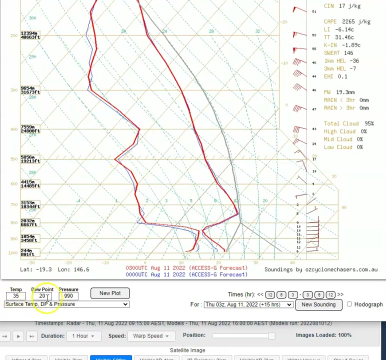 our potential for thunderstorms. This is why computer models sometimes get it wrong where in fact they've got it right. but they just don't realize that some slight temperature differences at the surface and dew point differences at the surface can make big differences in the in the actual atmosphere. So what we can do is we can manipulate these temperatures down. 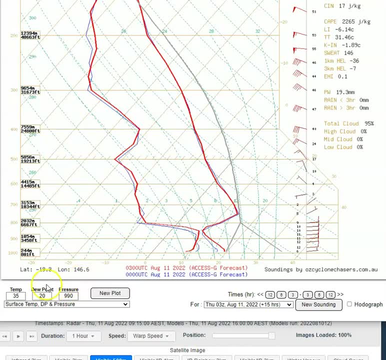 here We can use the ones that come standard with the model or we can change them based on what we've recorded. So a lot of us have weather stations at home and we can change these temperature and dew point values to reflect what we see on the weather station. So these are surface temperature. 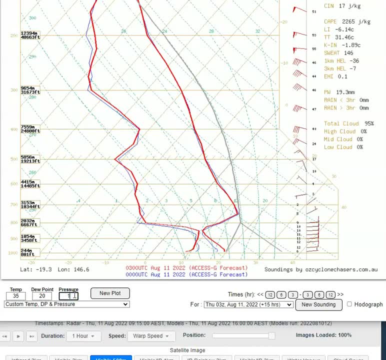 and dew point, and obviously we can change the pressure too. So it might be a thousand, a thousand and nine where you are, instead of 990, which is the model pressure. So what we can do then, and every time we change this, we can plot a new plot here and that will. 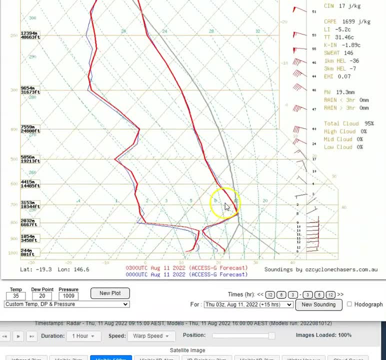 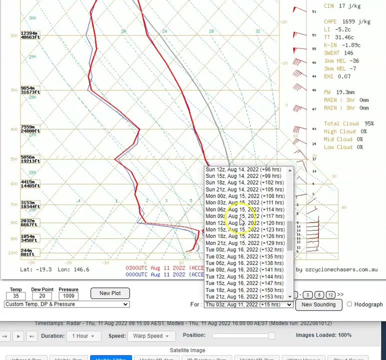 change the end result of what comes up here, what comes up here and, and what the potential is for rainfall. Now, on top of that, here we have, not only can we just move three hours, six hours or 12 hours forward or backwards, we can also change all the way through using a drop down menu. So, rather than 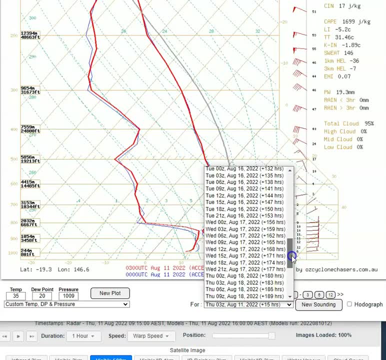 having. so let's say I'm looking at day one and I want to go all the way to day 10.. That's going to have to click the plus 12 hour thing 10 times. So rather than doing that, I've got a drop down and I 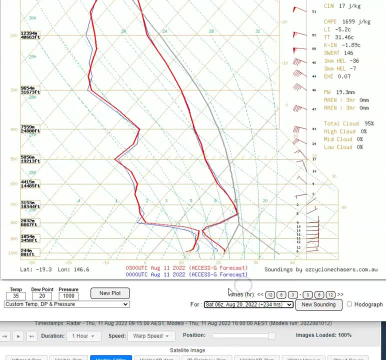 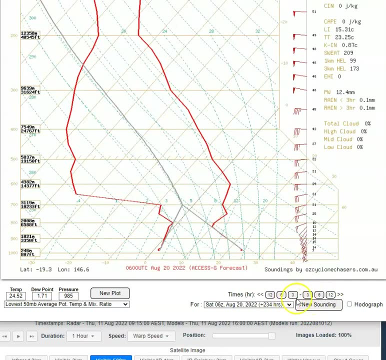 can go all the way to say Saturday at 4 pm, So Saturday 06 Z, And then I click new sounding and once again I have a new sounding here for Saturday at 4 pm and once again we go back to the model values here. So if I want to use my own values once again I 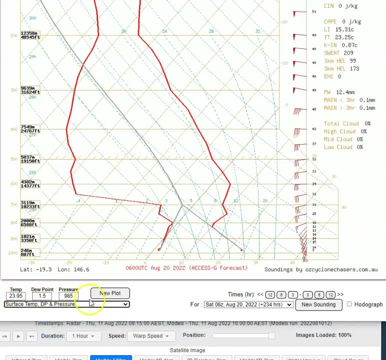 would change this to surface temperature and put in my own numbers in here of our our soundings, is what we call a hodograph. a hodograph shows us what the winds are doing at different levels of the atmosphere and they can reflect what, where, which direction storms could. 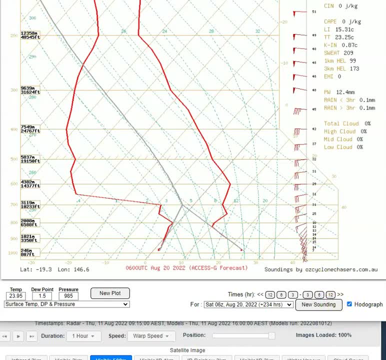 be moving in. now we've obviously got storm charts that do that, that show us the direction that storms should be moving in. but a hodograph is probably a more localized version of those of those maps that we have on the weather center model data. so what i would do here is i would 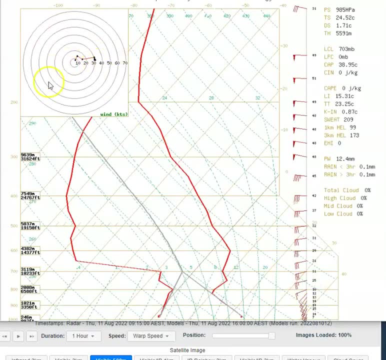 click hodograph and i would click new sounding and now what we've got is the sounding. so we've got the sounding, plus now the hodograph which shows us that if we were to get a thunderstorm today, on this particular day- which we won't because it's too dry and stable- we would see it. 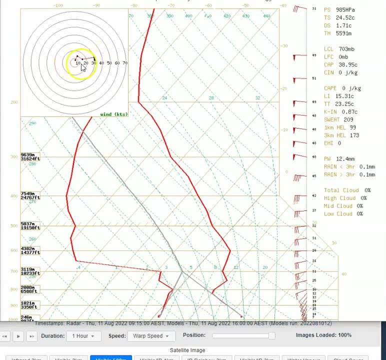 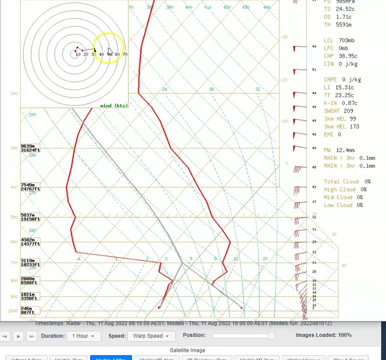 move from west towards the east, so in that direction, at around about 20 to 30 knots, would be the general, uh, the general, uh, you know- motion of that storm. so that's what a hodograph shows us, is what the uh different levels of the atmosphere shown here by the little. 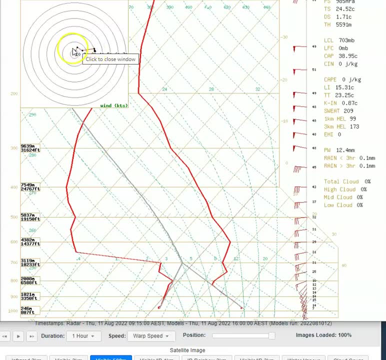 the hodograph shows us is what the different levels of the atmosphere shown here by the little black dots are doing and where those winds are coming from. and obviously, if we see something that's highly sheared, so something that's moving in a southwest to southeast direction, that sort. 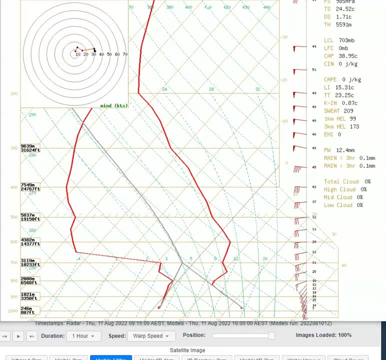 of hodograph. so if we're looking at something, for example, that looks like this, then we're looking at something that's really really super cellular or really intense, potentially from a thunderstorm perspective and in a tropical cyclone. i like to use these just because we 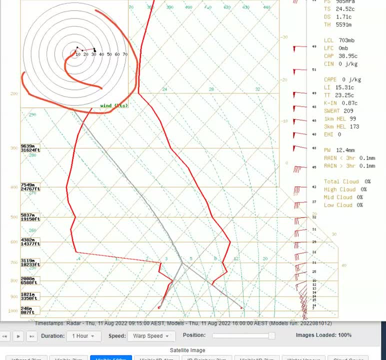 see hodographs that are way out here, sometimes completely off the charts. they're pretty crazy stuff. uh, well, sorry, they won't be like that. they'll be like this. uh, they'll be like- uh, let me just draw it in. so in a cyclone they'll be like that, and and the, the. 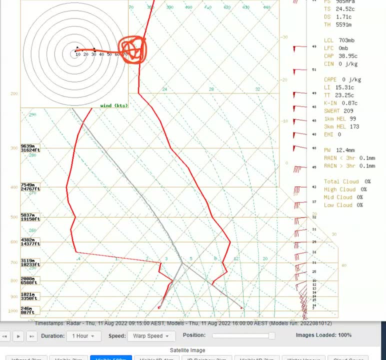 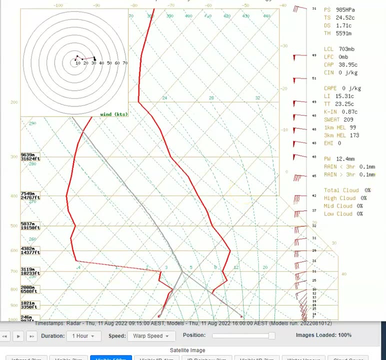 entire hodograph will be like that out here, around 50 to 70 knots. it'll be uh pretty crazy stuff, but anyway, that gives you an idea of what the different opportunities are for a sounding. now, remember, soundings are not a novice thing, they're not a basic thing if you're just getting into, uh the 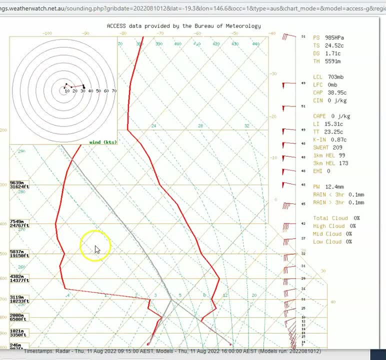 weather center and you're just learning the roads. and you're just learning the roads and you're just learning the slopes. this is not a tool for you. this is a tool once you get advanced on using computer model data and you want to start looking more at cross-sectional data of what the atmosphere. 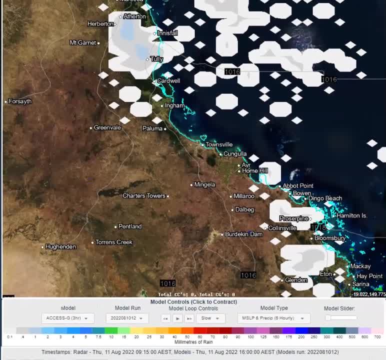 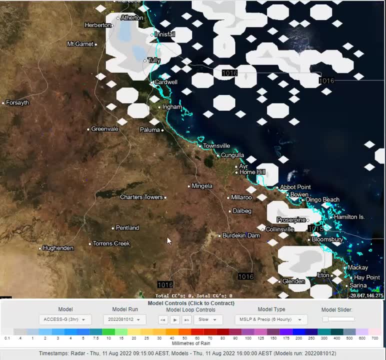 is doing. that's when we use the- uh, the soundings. soundings are a really, really important tool if you're a storm chaser, if you're chasing thunderstorms or if you're a really interested farmer that wants to start to really develop their knowledge on soundings and what they can. 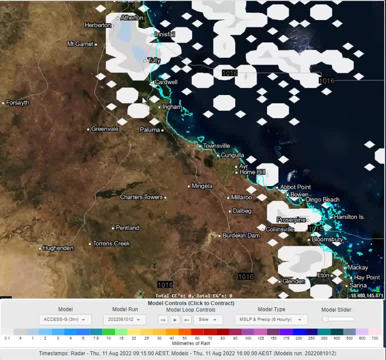 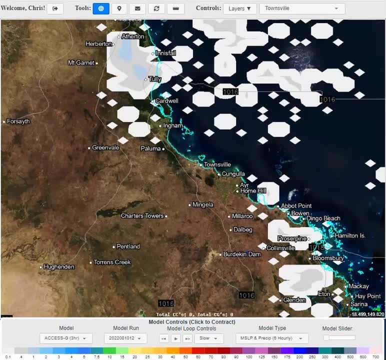 represent in the atmosphere. definitely start using those soundings and you'll be able to use those much more. this is a really advanced. this is the most advanced tool we have on the acc weather center and, as i say, you need to be fluent first at just normal model data before. 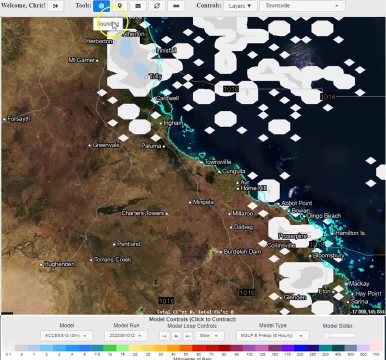 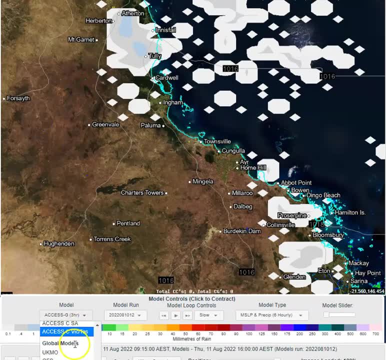 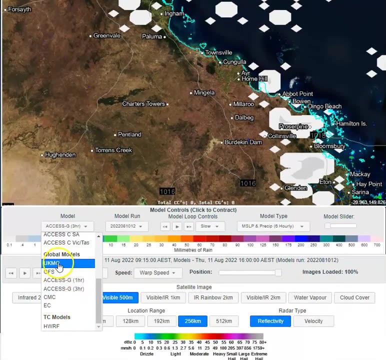 you start to delve into cross-sectional model data, like you're getting sounding. so soundings are available on the access, on all the models, the access c model- uh, for all the local models, and then also we're allowing uh, those, uh, those uh soundings for the euro. the access g. the gfs and the uk met. 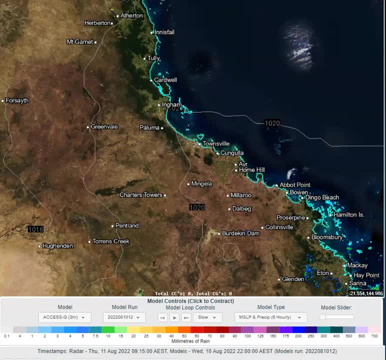 not have sounding data. just a reminder: there is a full soundings tutorial done by a good friend of ours, anthony cornelius, meteorologist from weather watch, and there are links to those step by step instructions on how to deal with soundings. that is your best, best, it's the best one i've seen. 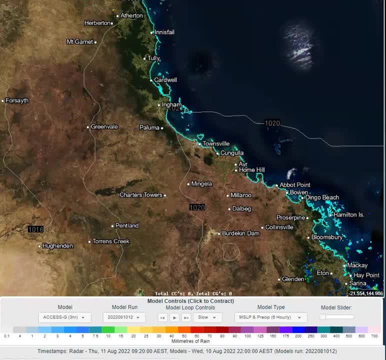 by far anywhere in the world. uh, tutorial on how to look at a computer model sounding. so if you're very, if you're already fluent in computer model data and then you want to take that next step in your journey and your weather, your weather intelligence journey, then you need to start. 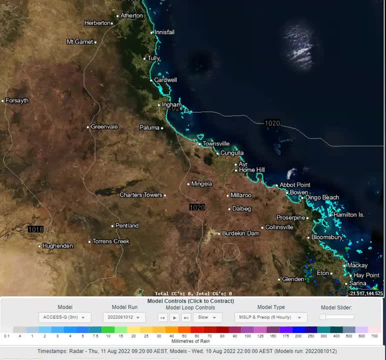 looking at that tutorial, which i've linked to just below this video. we hope you find the computer model data and particularly the sounding data that we offer on the acc weather center worthwhile and beneficial. thanks for watching.